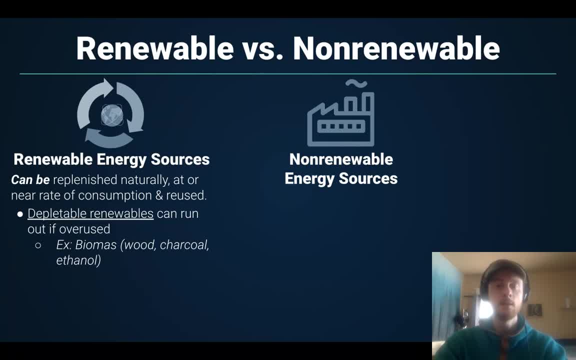 then we're not really using that sustainably and it does not exist as a renewable resource. It will run out eventually. Other examples are charcoal ethanol, which is a form of alcohol that we generate from corn. So if we're not replanting that corn and taking care of the soil in a way, 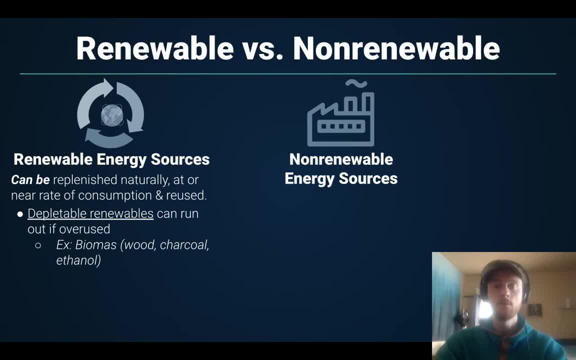 that's continuing to support ethanol production. we're not doing it sustainably and it's not a renewable resource. We have non-depletable renewables. These are renewable resources that do not run out when they're overused. They cannot be exhausted, And so examples include the sun. So if we put up solar panels, 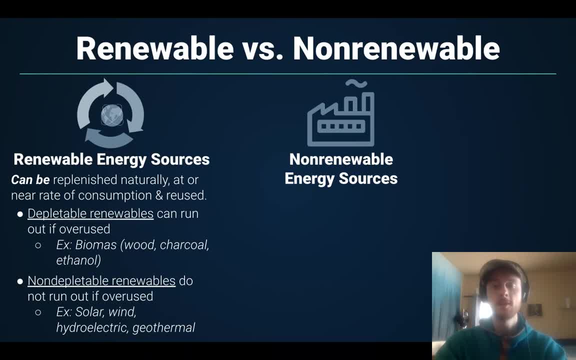 that doesn't make there less sunlight in the future. It's going to continue to shine. Same thing with wind turbines: We can harness the wind's energy. Wind turbines don't lead to less wind in the future. It can't be depleted or it can't run out. And then hydroelectric power as 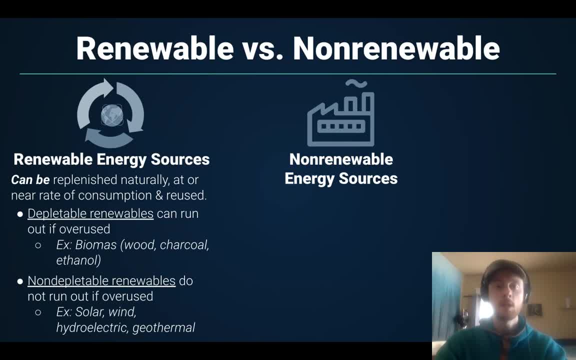 well, If we set up a dam in a river, we may cause some consequences to the wind, So we can't run out of the ecosystems nearby, but we're not destroying water. The water isn't ruined or depleted by its use for hydroelectric power. Non-renewable energy sources are depleted by their use and they exist. 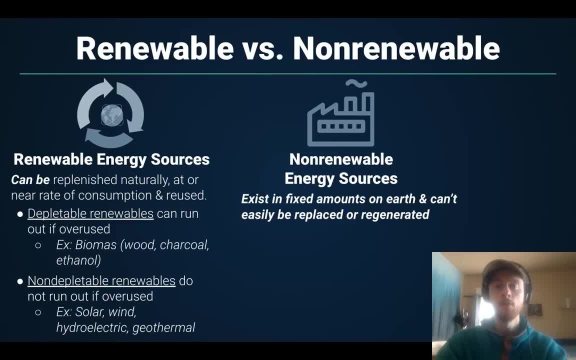 in fixed amounts on earth and they will run out when they're overused. So the best example is fossil fuels. These are the fossilized remains of biomass that get compressed under rock layers over millions of years, And that's the key: We're using them far faster than they regenerate. They 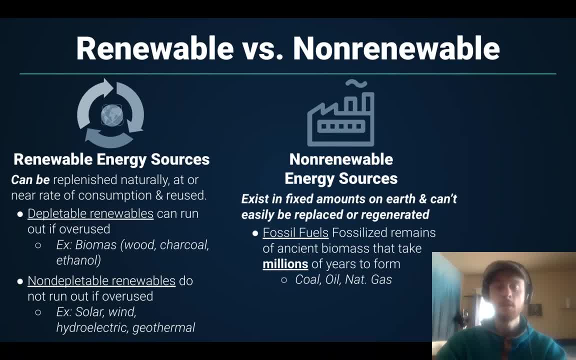 do not regenerate on any sort of time scale that humans can have access to, And so they're not renewable. They are coal, oil and natural gas. Unfortunately, they power the vast majority of our world's energy sources right now, And we're scheduled to run out of them in the not so 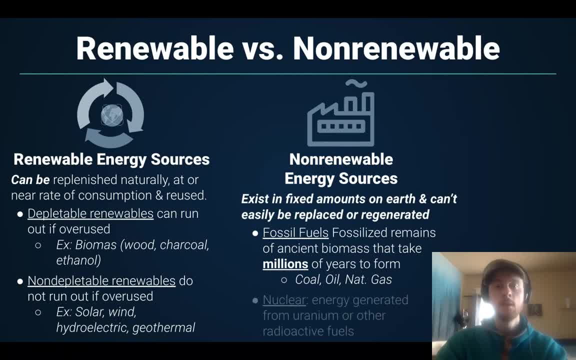 distant future. So these are non-renewable resources. Another non-renewable energy source is nuclear power. So nuclear power depends on radioactive elements, primarily uranium. but uranium exists in really finite amounts on earth And so it's also going to run out eventually. So the key to renewable 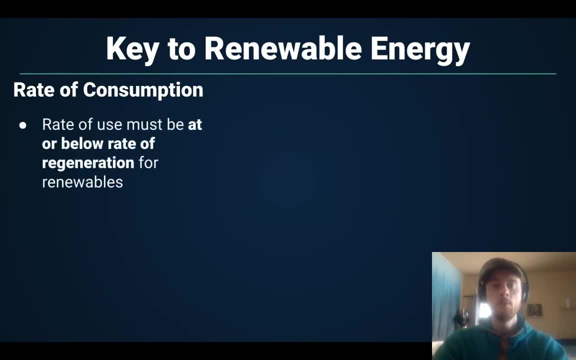 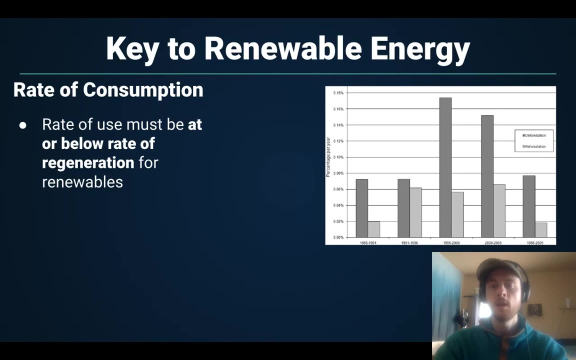 energy resources is the rate of consumption. We have to consume them at a rate that is at or below the rate that they regenerate, So we can't use them faster than they replenish themselves. This graph will show us an example of doing just that. In the dark bars we have deforestation.